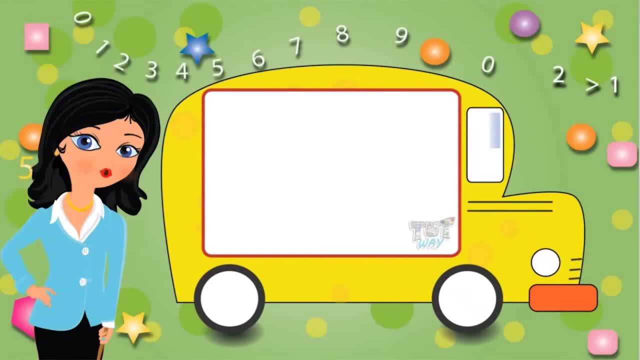 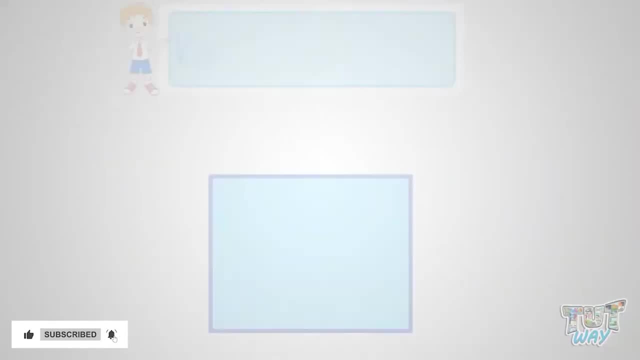 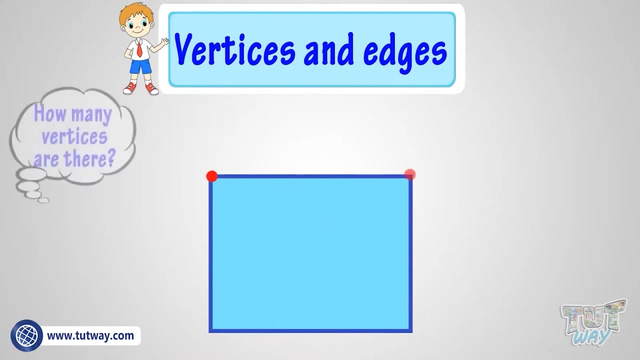 Hi kids, Today we will learn what are vertices and edges. The point where two or more lines meet is called a vertex. Also, vertex is a corner. See the vertices here in this figure. How many vertices are there in this figure? Yeah, Four vertices. Now, what are edges, Edges or sides? 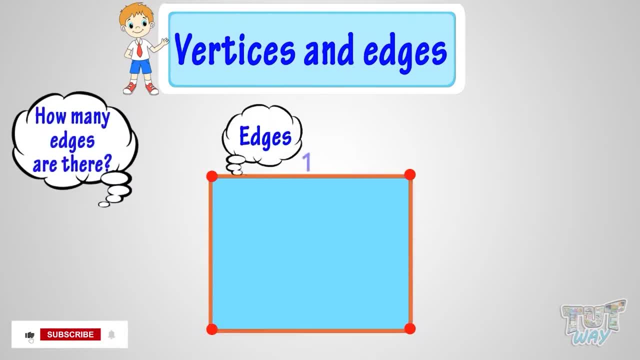 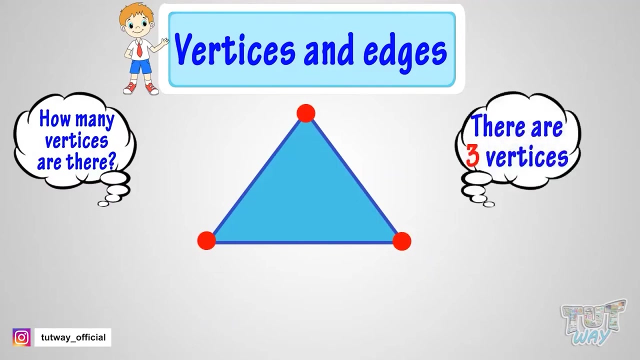 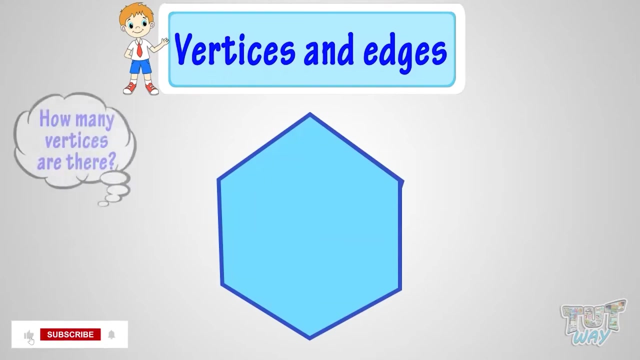 are the lines joining the vertices. How many edges are there in this figure? Yeah, Four edges. Good, Let's take more examples. How many vertices are there in this figure? Yeah, Three vertices. How many edges are there in this figure? Yeah, Three edges. Now here we have another figure. Let's see how many. 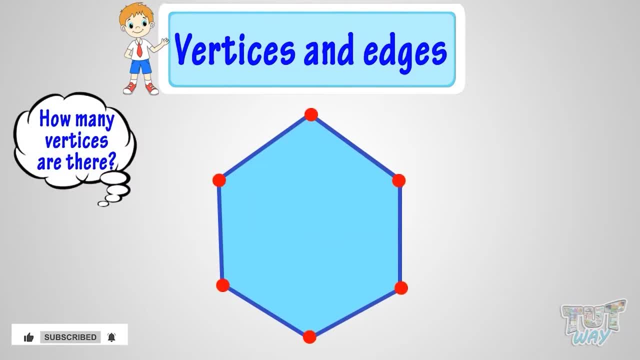 vertices are there in this figure. We know vertices are the points where two or more lines meet. How many vertices are there in this figure? Yeah, Two edges meet, or they are the corners in the figure. So let's count. One, two, three, four, five, six, Six vertices are there in this figure. 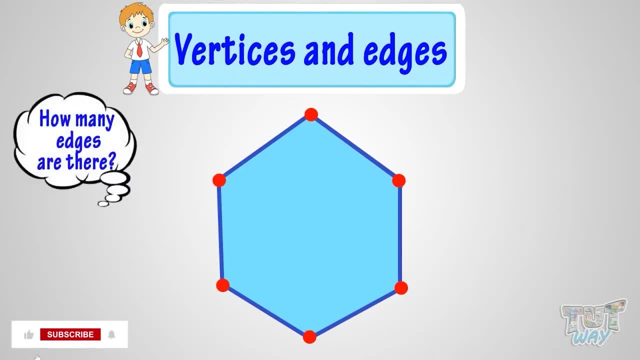 Now let's count the edges. We know edges are the lines. that joins two vertices count one, two, three, four, five, six, so six edges are there in this figure. now, here we have another figure. let's count its vertices and edges. we know vertices are. 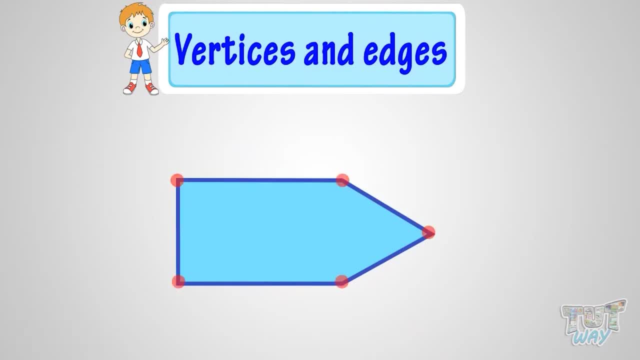 the points where two edges meet, or they are the corners in the figure. so let's count one, two, three, four, five. so there are five vertices in this figure. now let's count the edges. we know edge is the line that joins two vertices. let's count the edges one, two, three, four, five, so there are five edges in this figure. 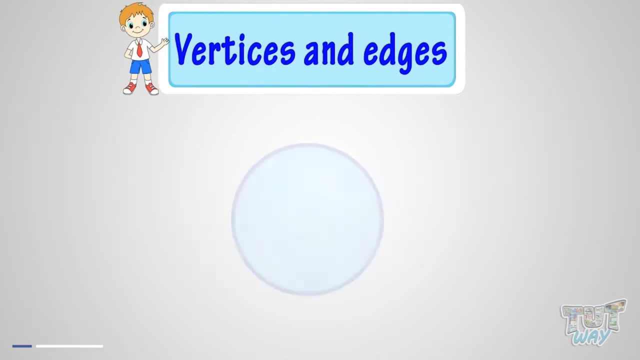 here we have one more example. let's see how many vertices are there in this figure. we know vertices are the points where two edges meet, or they are the corners in the figure. so let's count. oops, there is no corner in this figure where two lines or two edges meet. so there is. 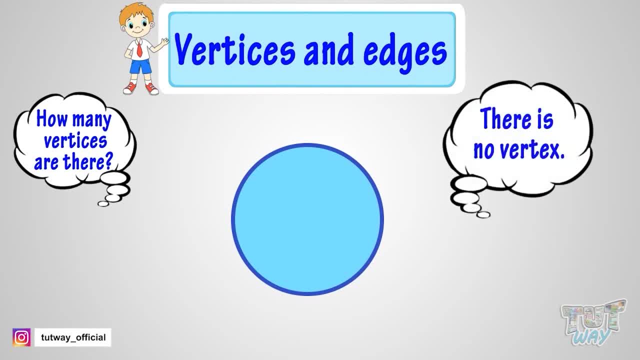 no vertex in the figure or no corner in the figure. now let's count the edges. we know edges are the lines that join the vertices. let's count: there is only one continuous line in this round shape that does not end anywhere. so this figure has one edge which is round in shape. so what would that be? 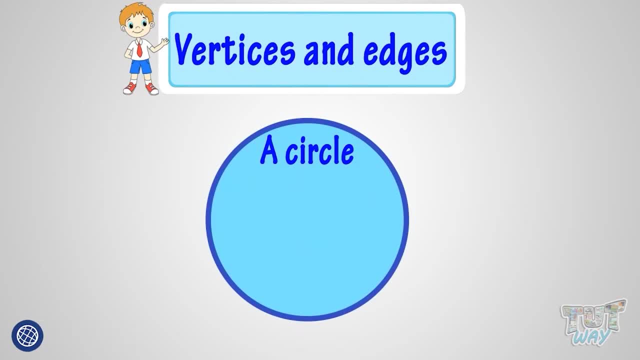 what we learn here. a circle or any round shape has no vertex and only one edge, which is continuous line that does not end anywhere. oval is one another shape that does not have any vertices and only one edge. so, kids, today we learned what are vertices and edges. now, you may go ahead and take a quiz to learn not only the edges of the circle but the end of the vertical line of the circle. so, kids, today we learned what are vertices and edges. now you may go ahead and take a quiz to learn. neither of these simple exercises we learned. 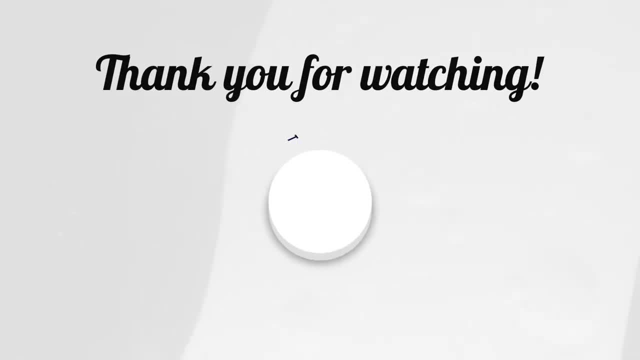 Thank you so much for watching. don't forget to like, comment and share this video, And if you want to see more fun videos, you can hit that subscribe button. You can also follow us on Facebook and Instagram for more content. Bye, bye.